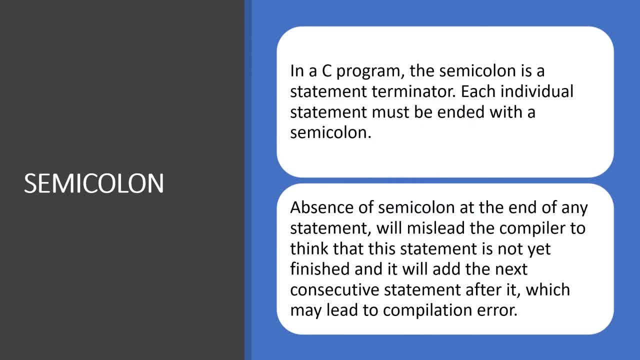 is a statement terminator, each individual statement must be ended with a semicolon. absence of semicolon at the end of any statement will mislead the compiler to think that this statement is not yet finished and it will add the next consecutive statement after it, which may lead to compilation error. 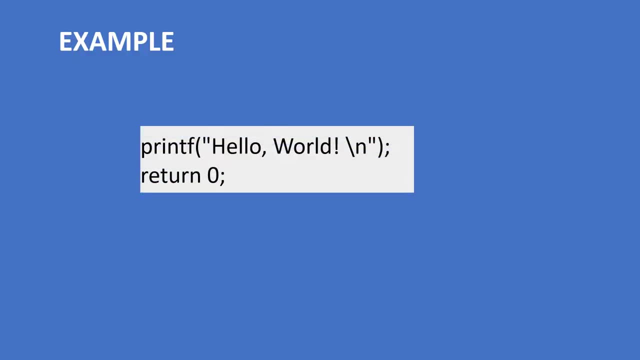 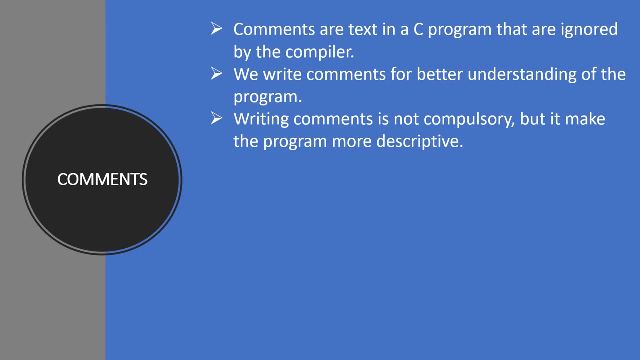 example. in this example there are two different statements. this is statement one and this is statement two. comments: comments are text in a C program that are ignored by the compiler. we write comments for better understanding of the program. writing comments is not compulsory, but it make the program more. 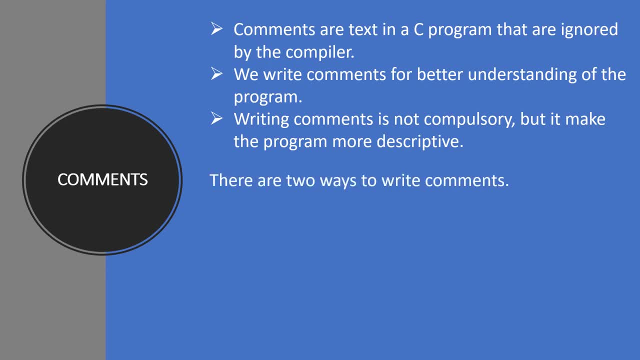 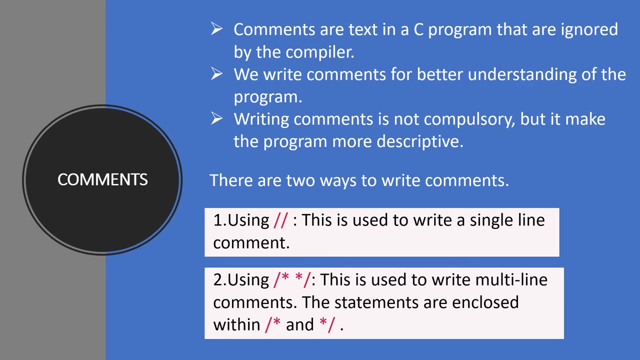 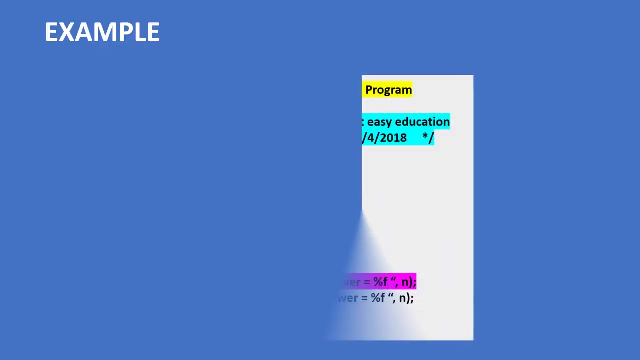 descriptive. there are two ways to write comments. using two forward slash: this is used to write a single line comment. using for slash star and star forward slash: this is used to write multi-line comments. the statements are enclosed within this example. this is a single line comment. this is multi-line comments if we want the compiler to ignore any statement. 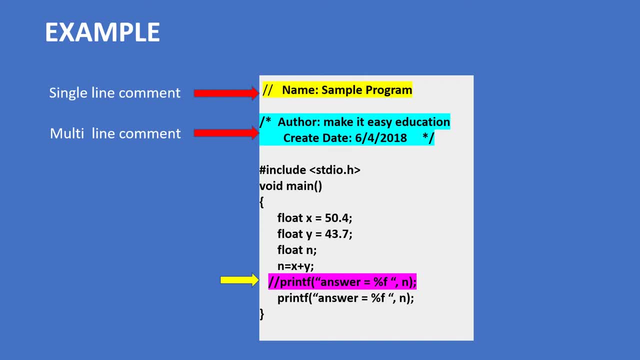 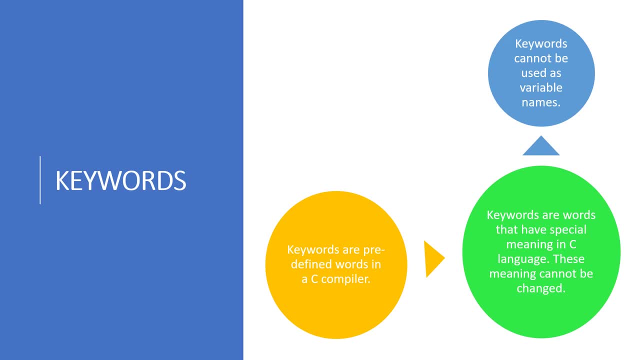 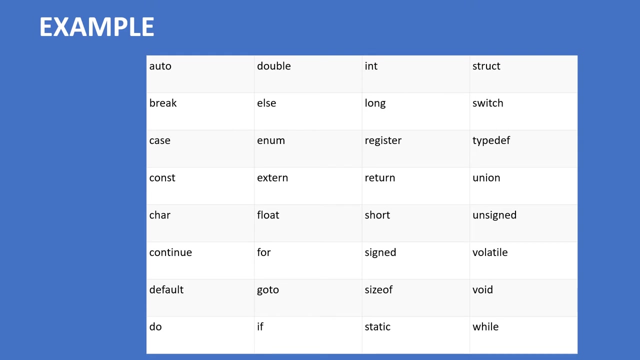 inside the C program. then we can do like this: keywords- keywords are predefined words in a C compiler. keywords are words that have special meaning in C language. these meaning cannot be changed. keywords cannot be used as variable names. example: the table shows the keywords used in C language identifiers. 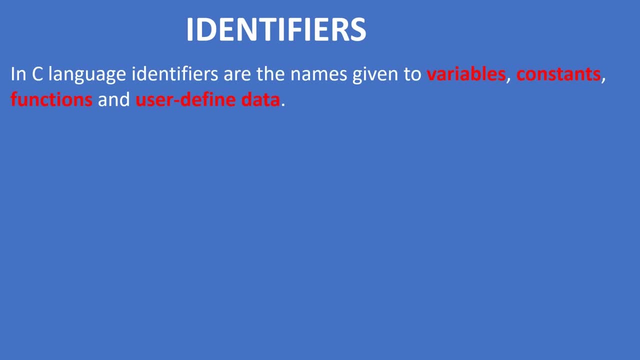 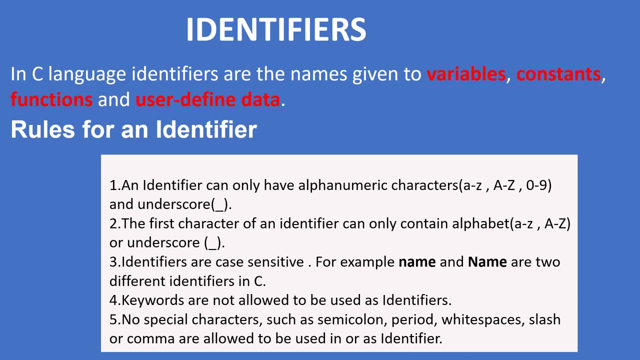 in C language. identifiers are the names given to variables, constants, functions and uses. you user-defined data rules for an identifier. an identifier can only have alphanumeric characters and underscore. the first character of an identifier can only contain alphabet or underscore. identifiers are case-sensitive. for example, name and name are two different identifiers in C. keywords are not allowed.